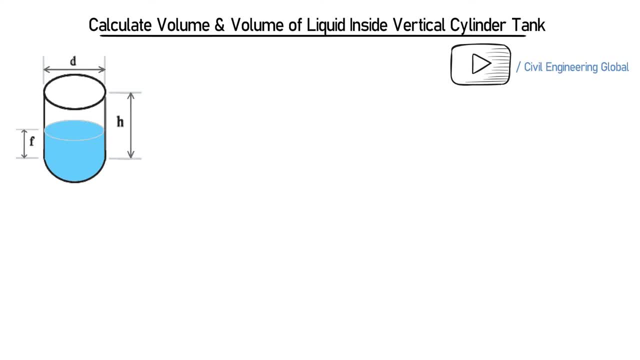 So, as we all know, the total volume of the cylinder is equal to area. this circular area multiplied by height and area is equal to pi r square For a circuit. So let's take an example. In this example we have the following data: 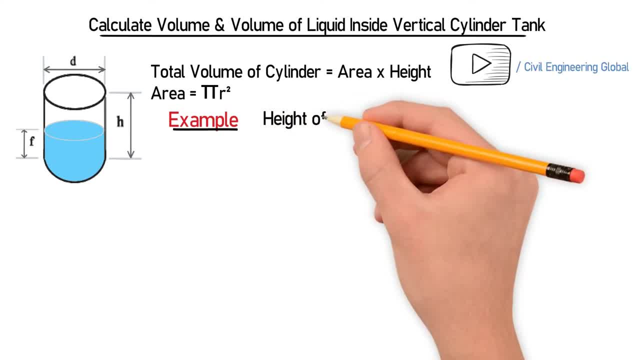 Height of the tank, H, which is 10 feet, Height of the liquid filled inside, F, which is 5 feet, And diameter D is equal to 10 feet. So radius r is equal to 10 feet. So radius r is equal to 10 feet. 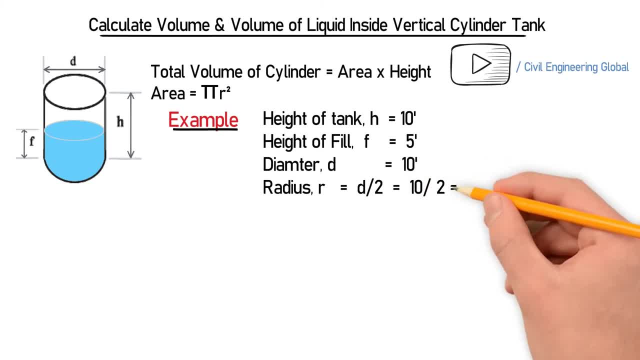 So it will give you 5 feet. So this is the data in this example. So let's calculate the volume of the tank. So to calculate the volume of the tank we have, the formula V is equal to pi r square multiplied by H. 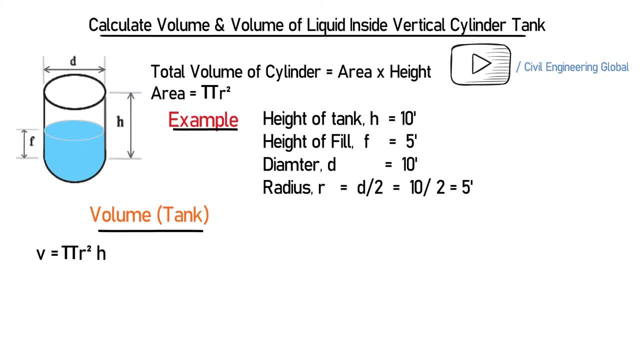 So, putting the values, we get 3.14. multiplied by 5 square, multiplied by 4. multiplied by height, which is 10, so this will give you the volume is equal to 785 cubic feet. so let's convert this volume into us gallon to you. to convert this into us gallon, you have to. 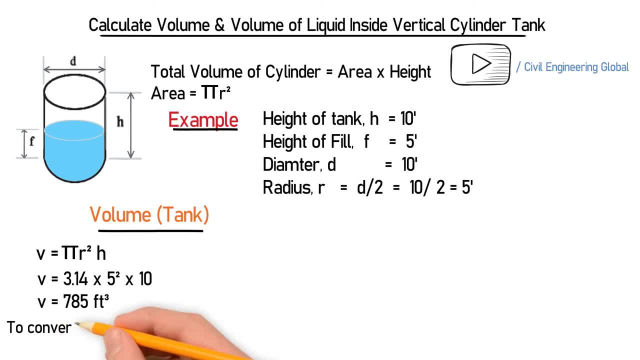 multiply it by 7.48 as 1, so to convert to us, gallon is equal to 785 multiplied by 7.48, which is equal to five thousand eight hundred and seventy five point nineteen. so this is the volume of the tank. let's calculate the volume of the liquid filled inside. so how much liquid is? 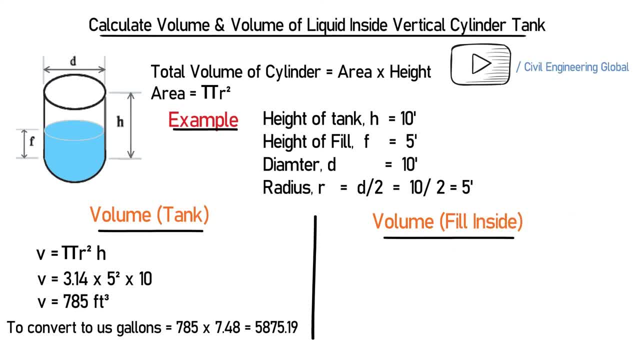 inside this tank. so for this we have the formula: V is equal to PI R square F. F is the filled height. so let's put the values we will get. V is equal to 3 multiplied by 1. 4 multiplied by 5. square multiplied by 5, V is equal to three hundred and twenty nine three.